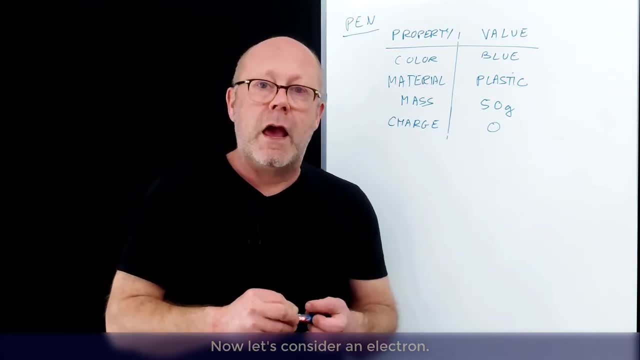 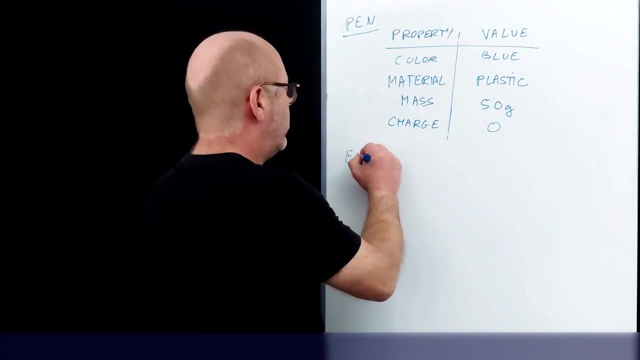 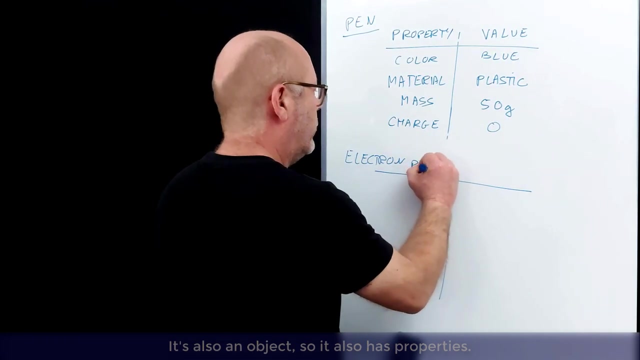 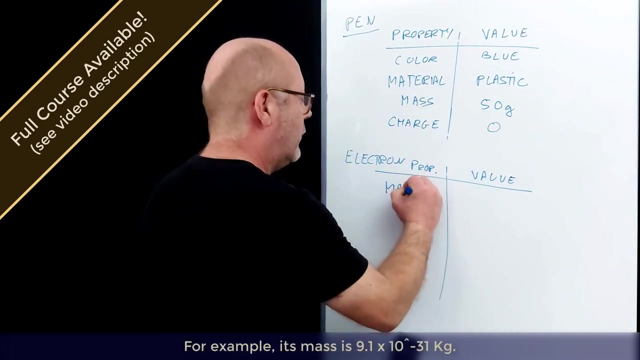 Now let's consider an electron. An electron is an elementary particle which is part of an atom Electron. It's also an object, So it also has properties And values associated with it. For example, its mass is 9.1 by 10 to the minus 31 kilograms. 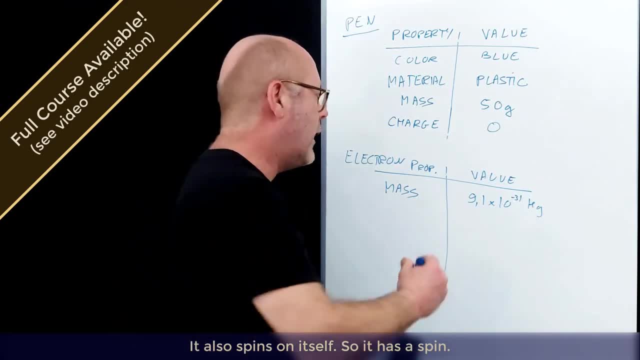 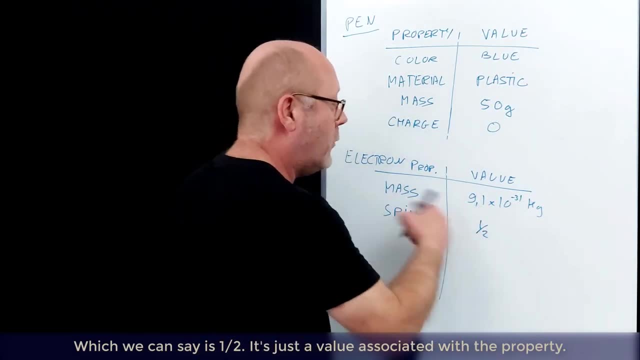 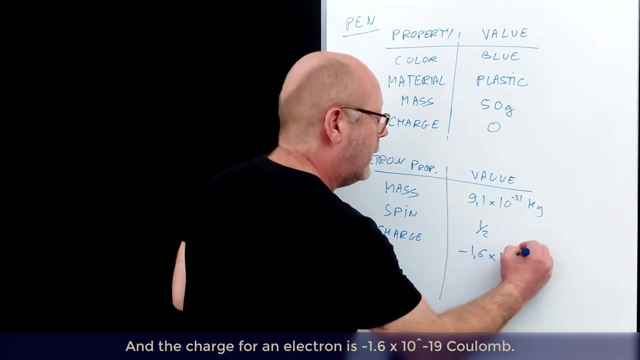 It also spins on itself, so it has a spin which we can say it's a one-half, It's just a value associated with a property. It also has a charge, and the charge for an electron is minus 1.6 by 10 to the minus 19 Coulomb. 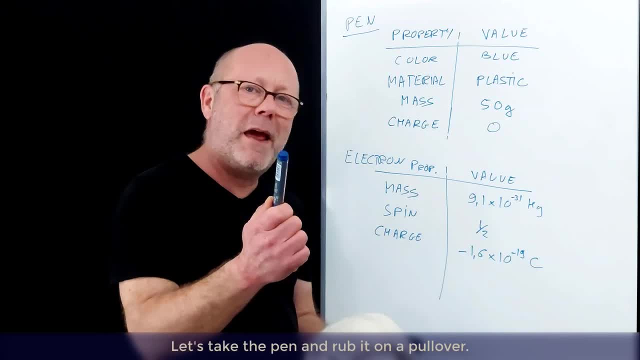 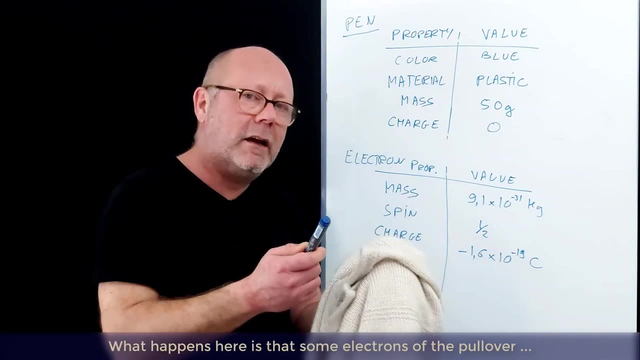 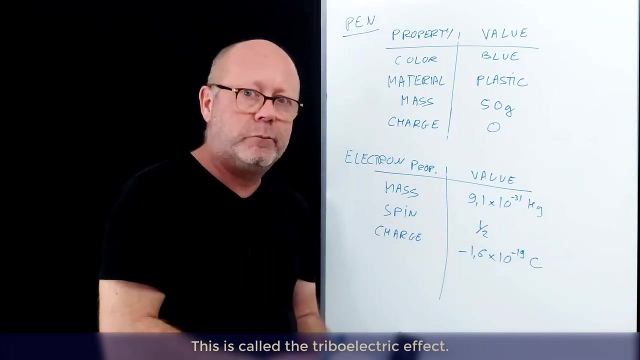 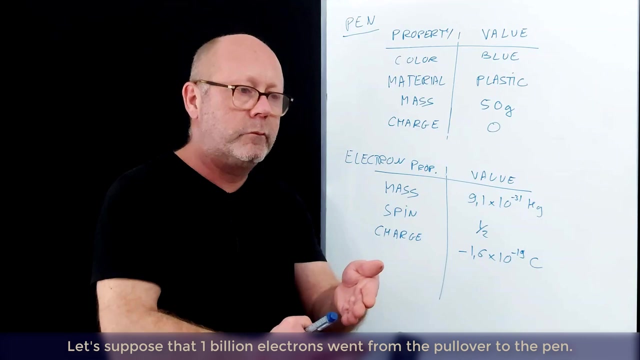 Coulomb is the unit of charge. Let's take the pen there and rub it onto a pullover. What happens here is that some electrons of the pullover are transferred to the pen. This is called the triboelectric effect. So now let's suppose that one billion electrons went from the pullover to the pen. 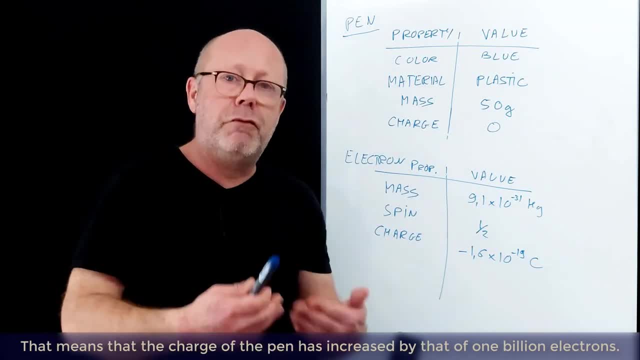 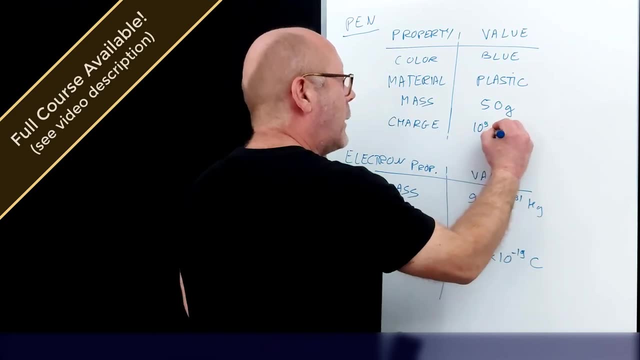 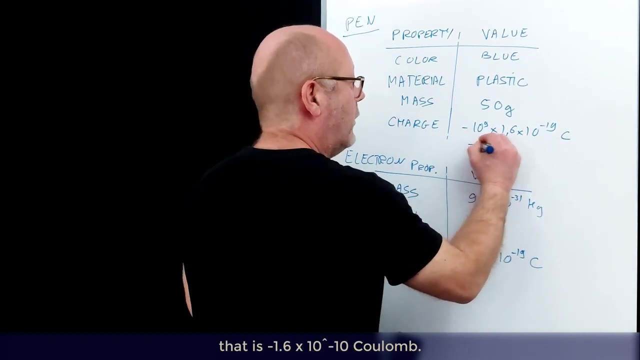 That means that the charge of the pen has increased by that of one billion electrons. One billion is 10 to the 9, that are multiplied by the charge of one electron. that is, 1.6 by 10 to the minus 10 Coulomb. 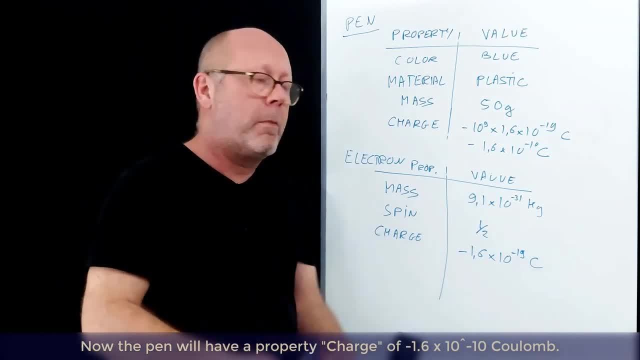 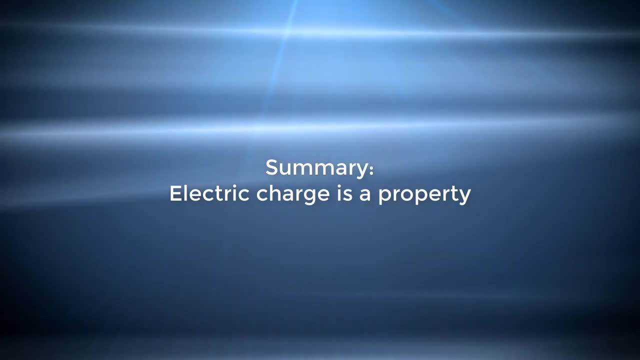 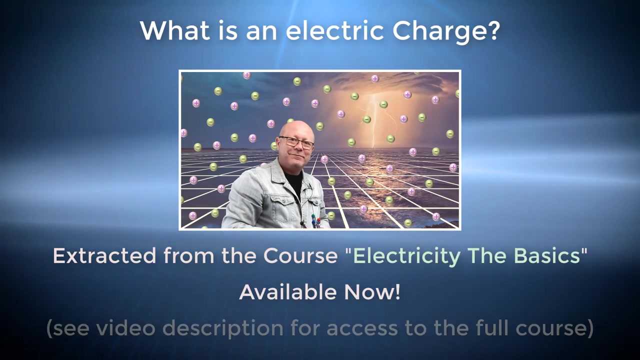 Now the pen will have a property charge of minus 1.6, 10 minus 10 Coulomb. What happens here is that it will have a charge of minus 1, 10 to the minus 9 Coulomb. That's what we're going to be doing here. 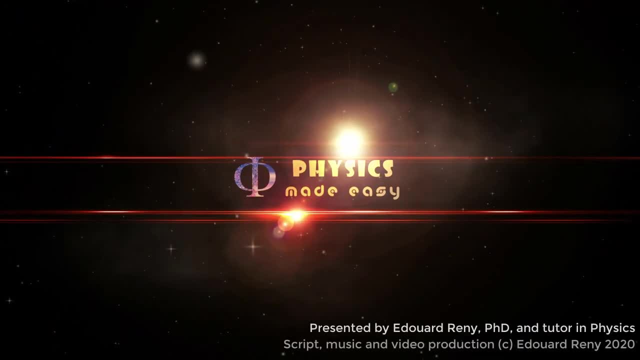 We're going to be giving the current number to the current number. The current number will be 10 to the minus 10 Coulomb. That's the current number we want to give to the current number.